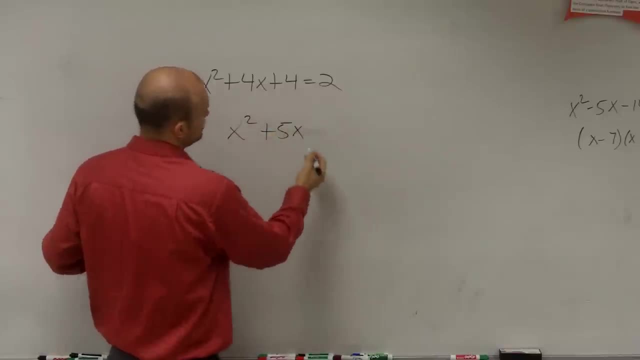 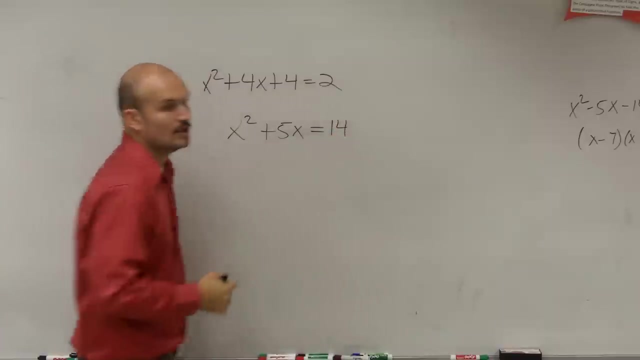 was my previous example- X squared plus 5x equals- I'm sorry, equals 14.. Okay, We had to solve this. What we always had to do is solve by factoring. We always had to get this equal to zero And the 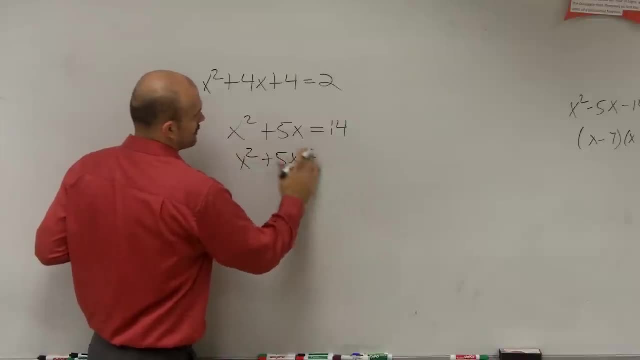 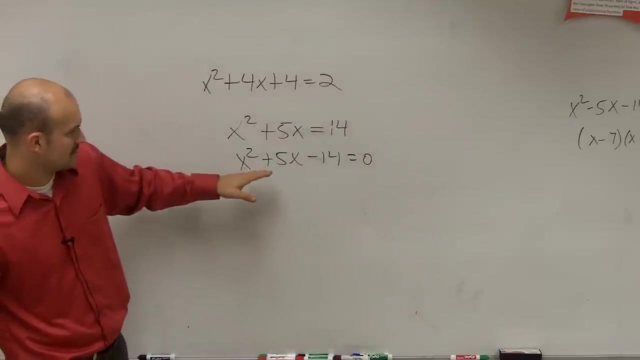 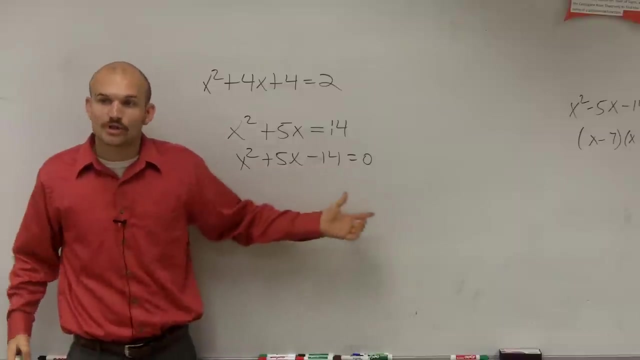 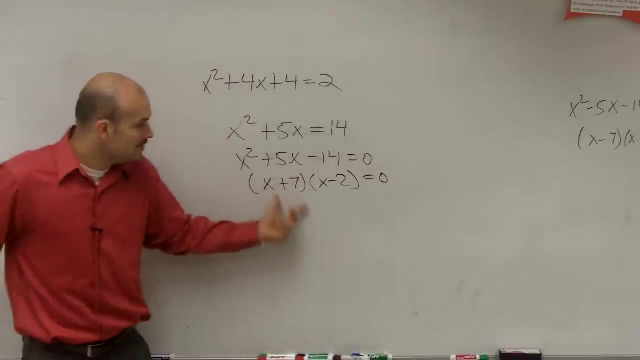 reason why is because when we learn to factor, okay, positive 7.. Okay, When we learn to factor, what we had to do is we had to set it as a zero product property. So we do our factor and we'd say: x plus 7 times x minus 2 equals zero. Only when we had 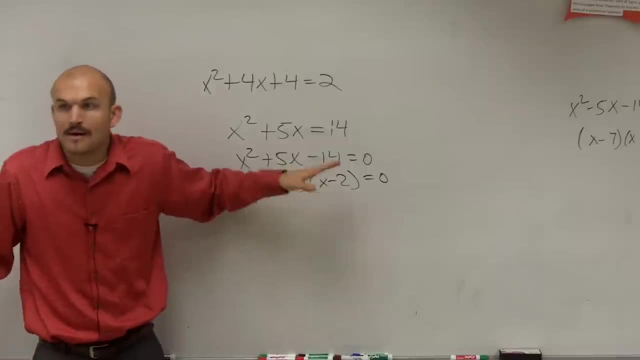 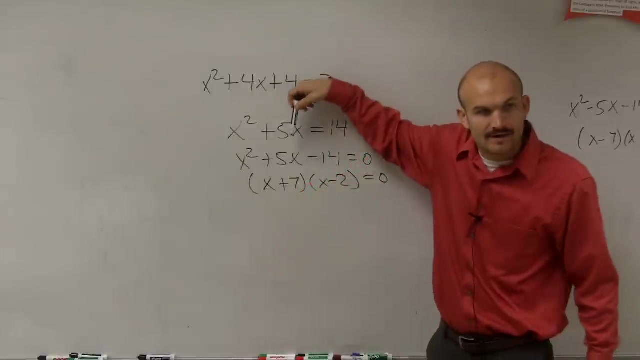 this point, could we say this equals zero or this equals zero by the zero product property? It is essential that you guys understand this, Sam, that you guys understand When we have a factoring problem and I say solve, I'm going to say okay, when we learn to factor, what we had to do is: 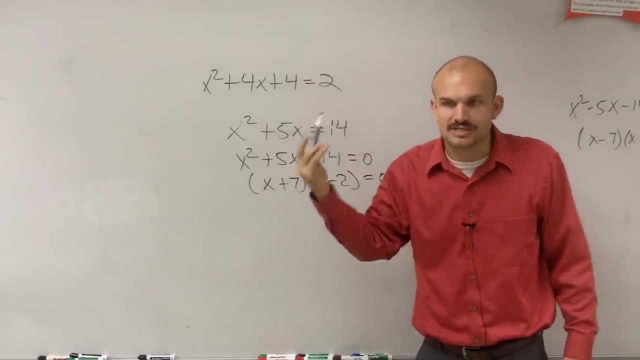 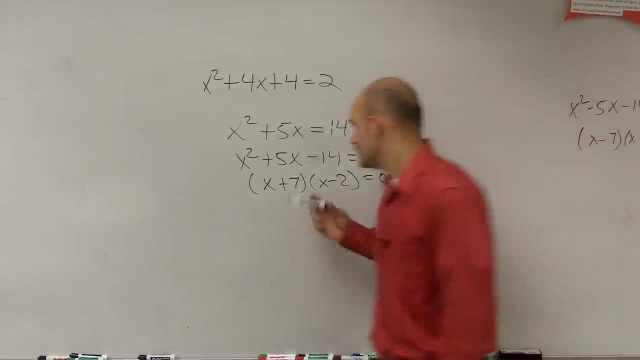 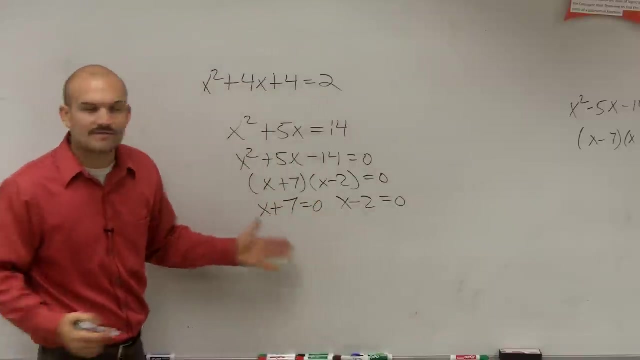 solve. You have to use factoring and you have to use the zero product property. You have to set it equal to zero, factor it and set each of those equal to zero. So therefore you could say: x plus 7 equals zero and x minus 2 equals zero. Now you can find the values of x that make that true X. 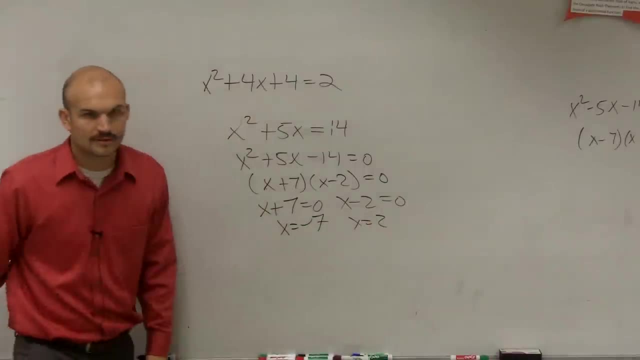 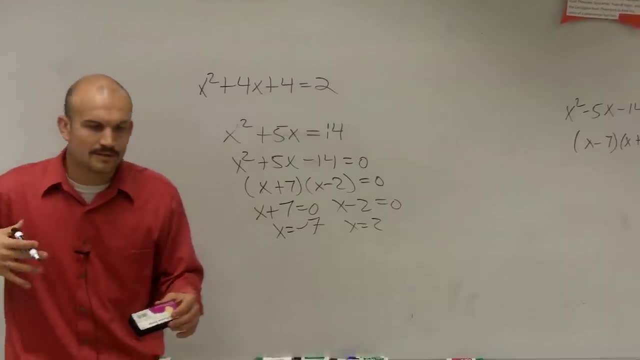 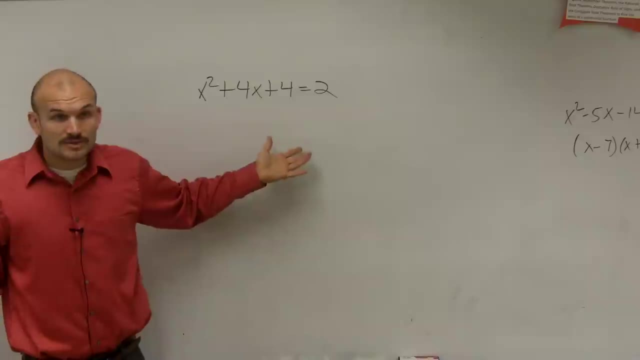 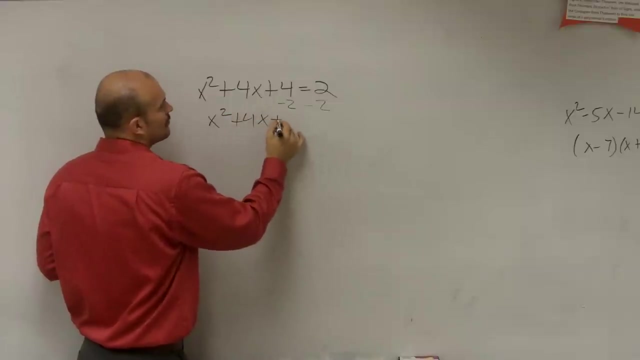 and almost natural for you guys to want to do that for this problem, because that's the way we've been teaching it- Say: hey, get it set equal to zero, right? So you do that. So you subtract two on both sides. So therefore you say: x squared plus 4x plus 2 equals zero. But then you come. 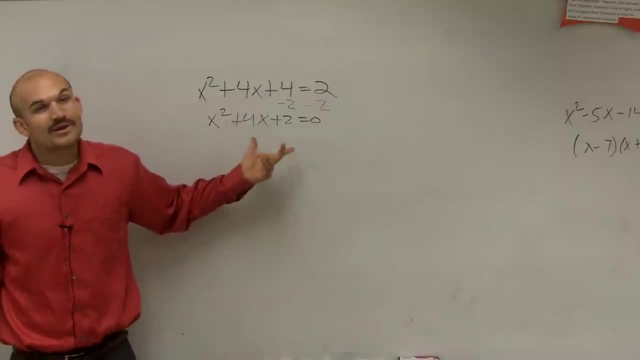 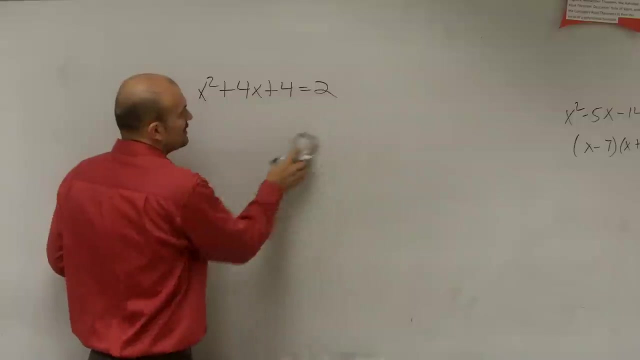 into a problem when you do that because is this factorable? No, it's not even factorable. So there's still ways we could solve it. but there's a trick, Kind of an easy way to look at this, and this is what you guys need to have your mind trained for. 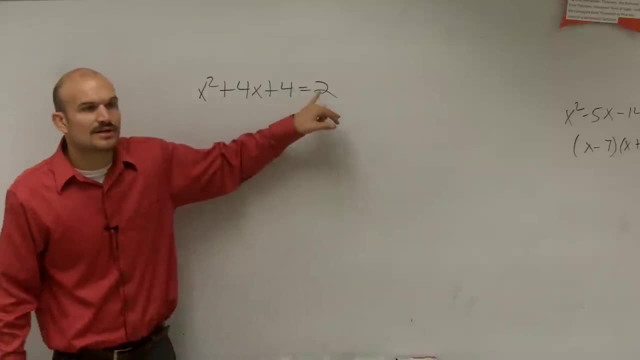 is looking for perfect squares. Remember, we always look at our last number and can we determine: is that a perfect square Or, I'm sorry, is that a square number? Yes, four is a square number. right, It's two times two. Then we say: is the square of that number? is that double?